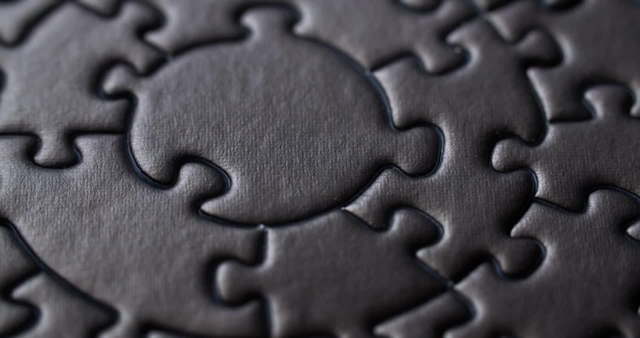 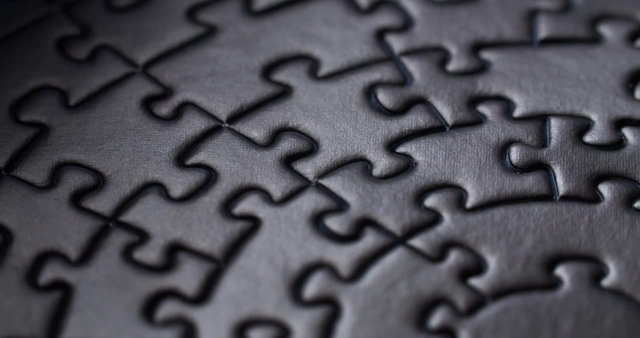 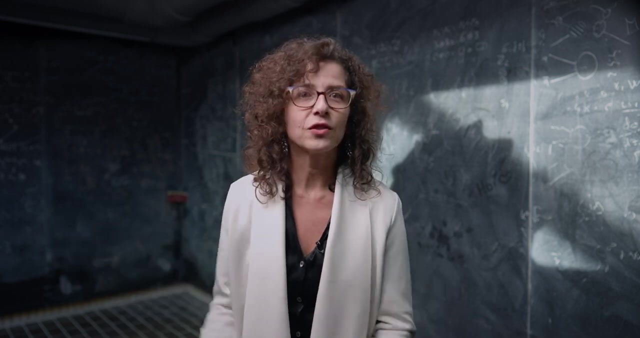 So it's like when you are constructing a puzzle that the pieces start to be put together and forming a big figure. So I study collisions between protons. that leads to the production of B mesons, B hadrons. It's a type of particle. 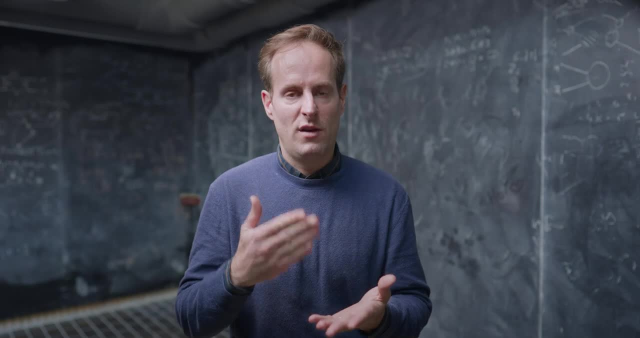 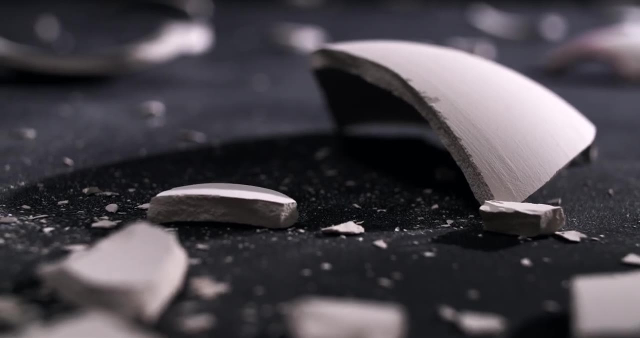 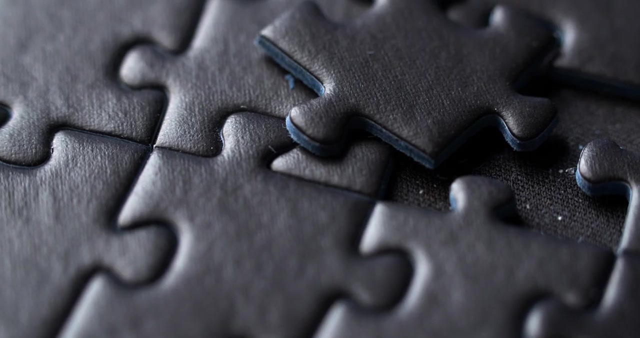 We have our best theory of nature, which is called the Standard Model of Particle Physics, And this makes very specific predictions. But these predictions have some uncertainty. When the puzzle is finally completed, it happened that there are some pieces at hand that do not fit the Standard Model. We have now a sample of B mesons decaying to some specific 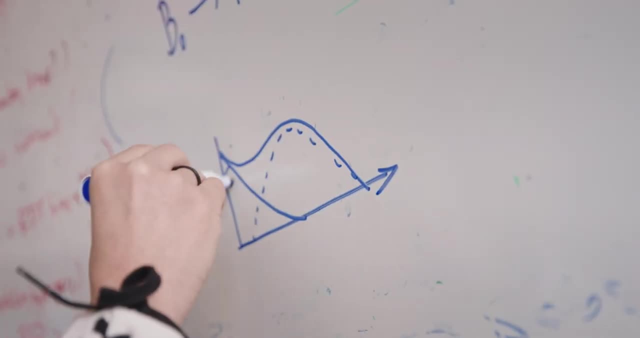 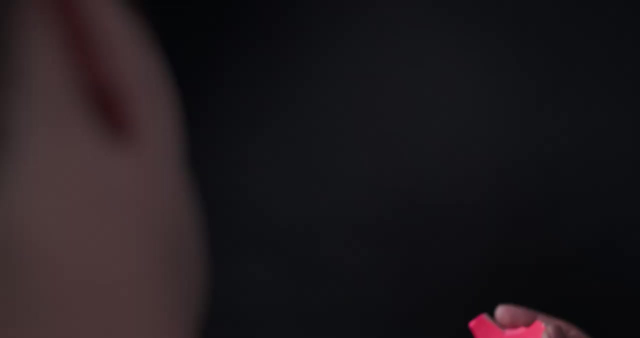 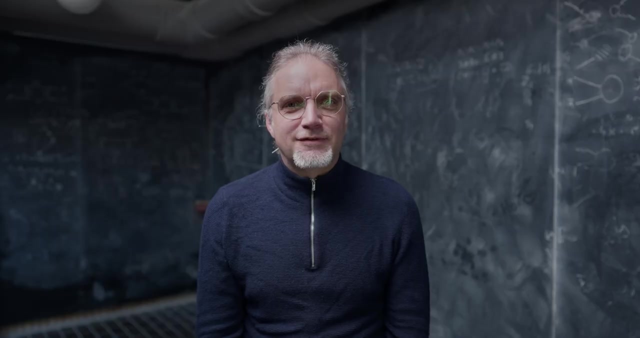 particles that simply do not fit the theory very well at the moment, And so there must be something else there. This big insight has been there waiting for someone to pick it up. if only someone asked the right question and with the right tools- A gravitation wave. it's ripples in space and time itself. This leaves echoes traveling. 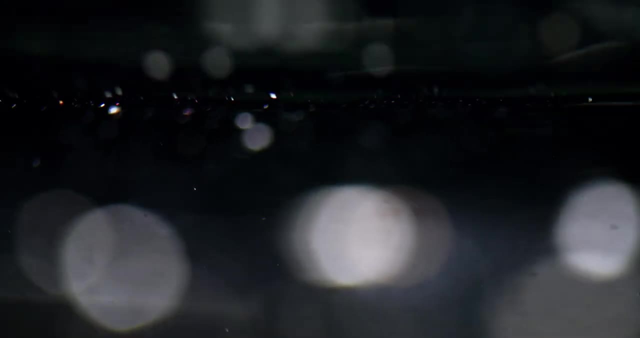 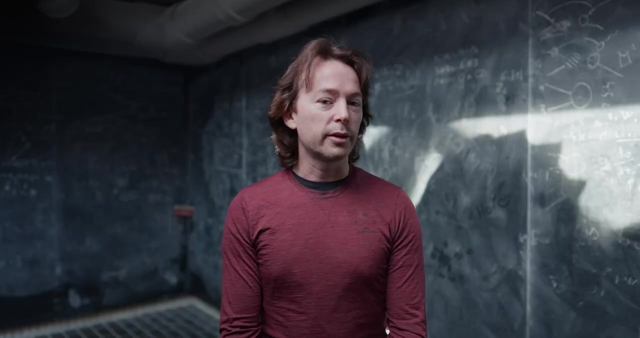 through space to us Objects that you cannot see with the normal visual light, And we capture that signal. And to do that we need to overcome a seismic wall. the noise we get from nature, This is the waves crashing on the seashore. 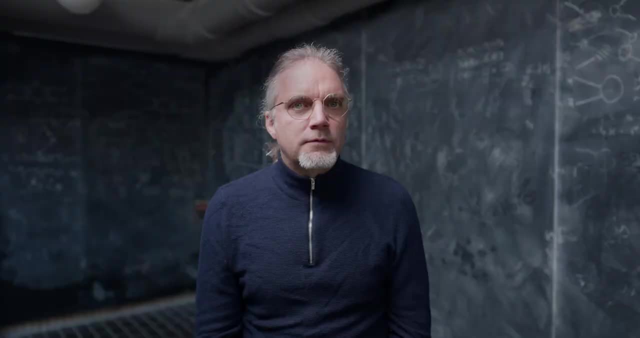 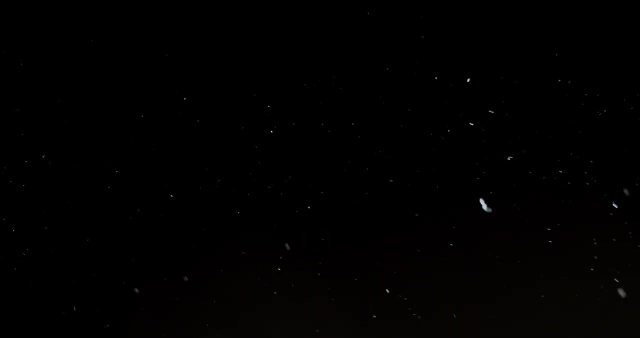 That's from people, People and cities. So we believe with our new instrument, the Einstein Telescope that we're going to build, we can go way beyond what optical telescopes can see, even into a region where we believe there are not even stars yet. 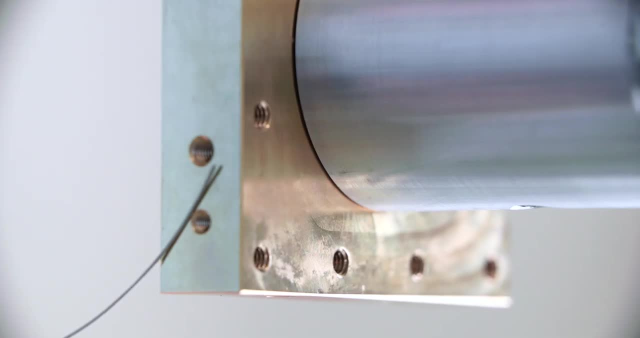 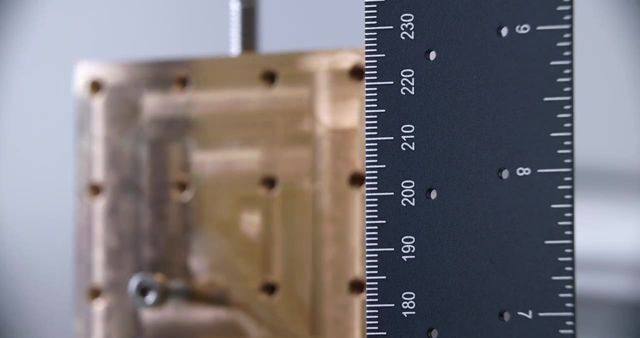 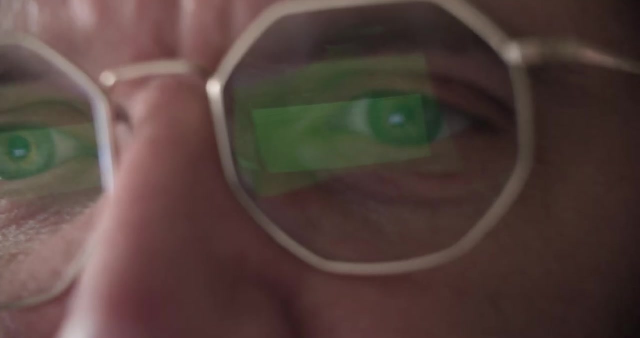 That lets us reach deeper and deeper into the universe to measure the collisions of all of the stellar mass black holes in the universe. So my work is really to look into the physics and then say, okay, what exactly do I need to model? I think model building is always. 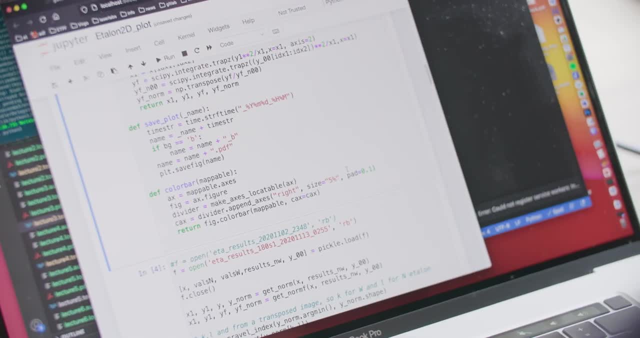 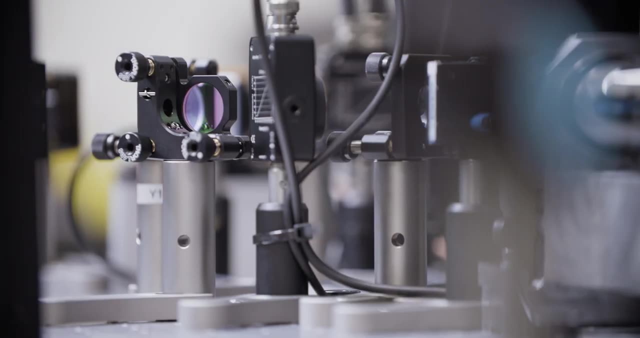 Making it simpler in exactly the right way. How can I do this in the computer in the best way? It's simpler than reality, but it's so complex that it can do all this kind of complicated physics, that we need the gravitation waves, the quantum optics, in the correct way And